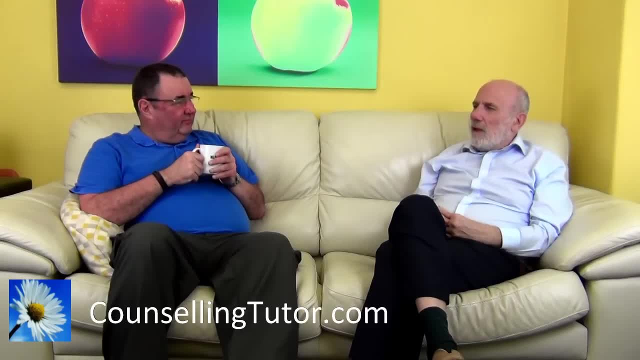 psychological literature developed um and today we've got object relations therapy um. Sheldon Cashton, who wrote one of the probably the most prominent book on object relations theory- stroke therapy came out with a book on 1990 where he talked about object. 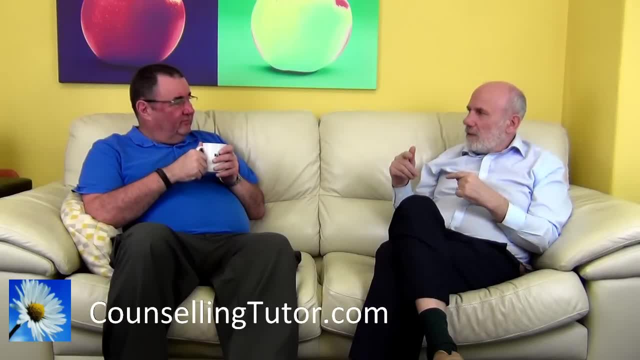 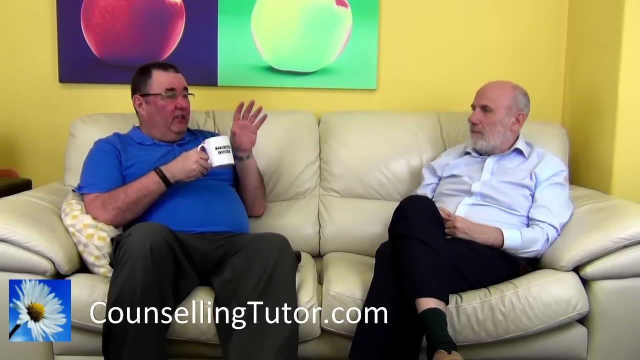 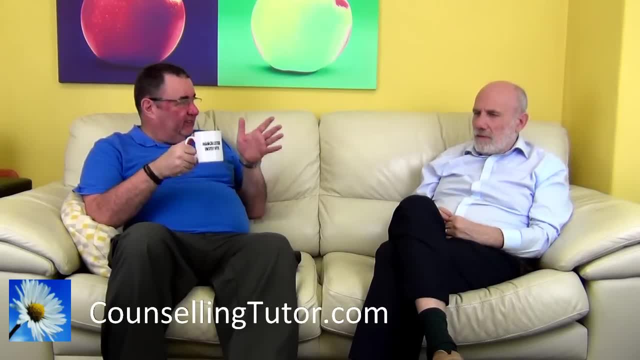 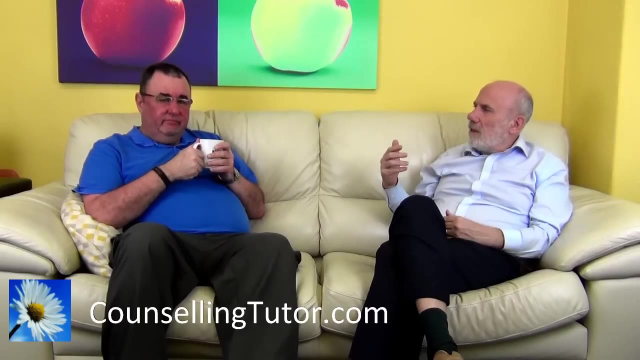 or a significant individual in somebody's life, Correct, And that's usually the term that we use when we talk about object relations therapy. So what happens is, in the development of the psyche, the child internalises the other, which is the object. 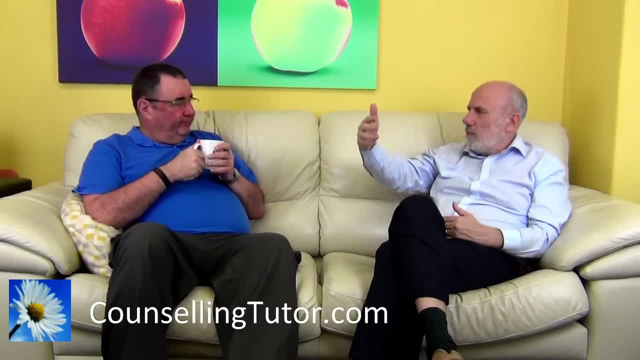 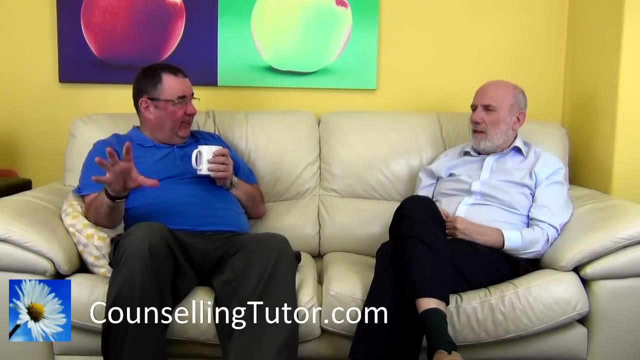 Right? So the mother, the father, the sibling, etc. Right? So if we look at the development of the child and let's look at psychodynamic development, So this is psychodynamic theory. This is really in the remit of the psychodynamic model. 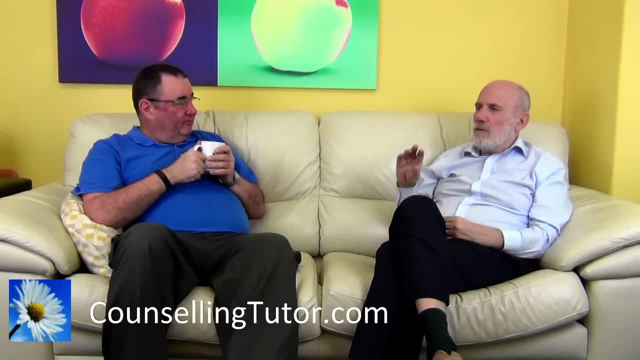 Margaret Marlowe. Right Now she talked about. one of the most important parts of child development is the time between one-and-a-half and three-and-a-half, which she called individuation separation period- One-and-a-half to three-and-a-half. 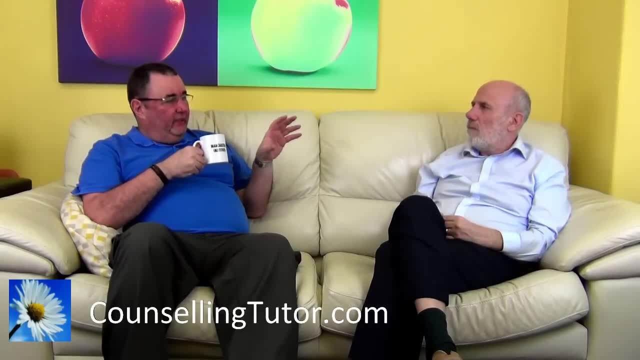 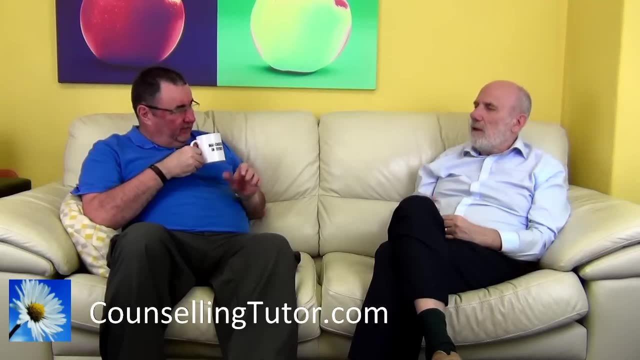 Okay, And that period would be where the child is becoming autonomous- maybe Correct. Yeah, starting to find their own life and their own experience. Yeah, And the major goal in the completion of this period is what Marlowe called object constancy. 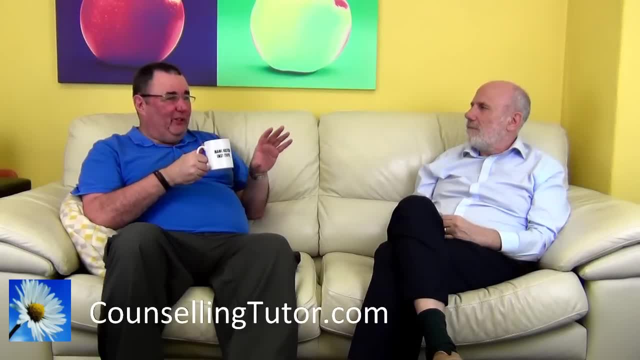 Right Now. I've done a little bit of study on this before I came today, which is always a dangerous thing- your little knowledge, But object constancy. I'm getting as consistent attention or caregiving, Correct Yes from the caregiver. Yeah, So you've internalised the constant mother. So, Margaret Marlowe, split up the individuation separation period into periods of what is called infant practising. So in the search for individuation or object constancy, the infant would practise throughout this time. 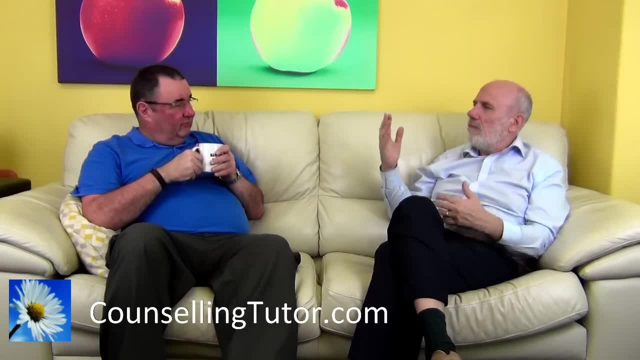 the movement away from the self in search of autonomy, Yeah, And then, at the same time, is internalising the object at a constant level, So that, in other words, the mother or the caretaker is always there in the psychological make-up of the infant. 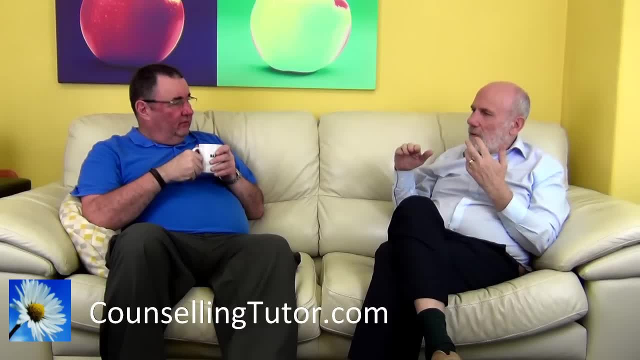 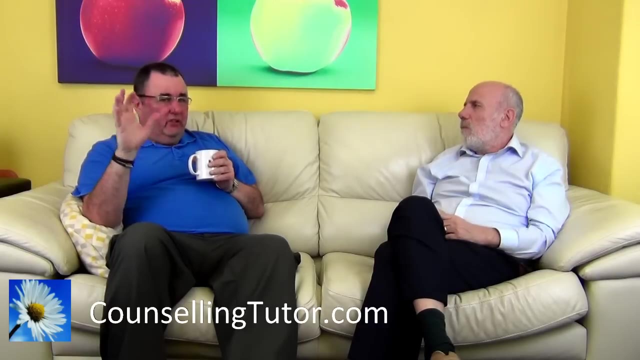 not only in constant you know, day, you know, but also in terms of stress. So under stress they have a constant internalised other in their head. Okay, So it sounds to me- I know we talked off camera earlier about the Jiminy Cricket character- this notion that as the child's separated, 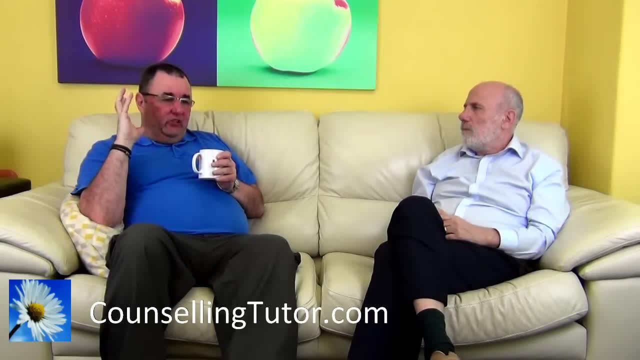 they carry with them a Jiminy Cricket character. If you watch Jiminy Cricket, he sits on the shoulder of Pinocchio, telling him the right thing, soothing and giving sound advice, and this sounds like the object you're talking about. It sounds like this is the caregiver. 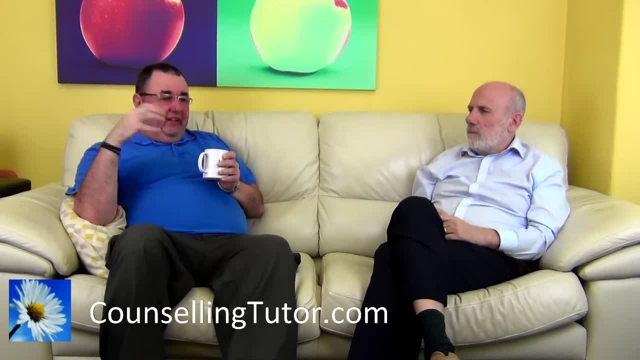 So when the child is under stress, then they revert back to that caregiver. It's almost like a mechanism of soothing Correct. A good enough other, A good enough other, And Winnicott's term for this is a good enough mother. 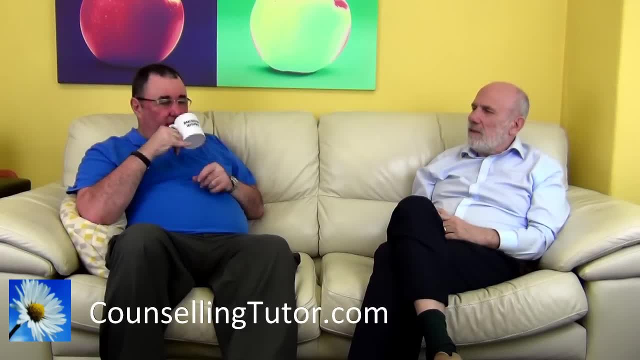 Right Now, of course, you internalise as well the father, the parent, the siblings, the immediate family In object relations therapy. it's that family that we're referring to Right. So when we're looking at specific therapy, object relations therapy. 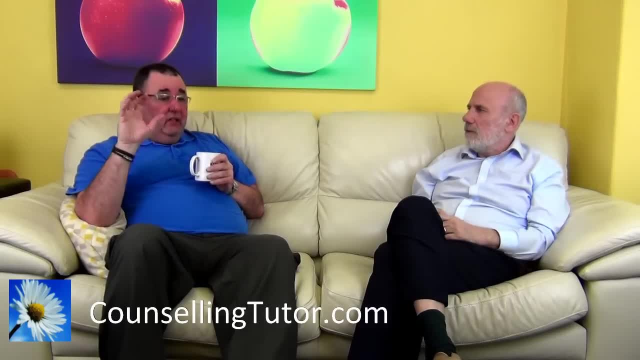 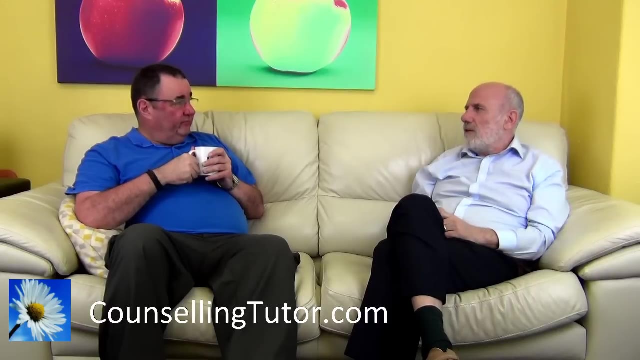 which is a specific type of psychoanalytic therapy, that the work would be about helping the client to identify initially what that caregiver was. Yes, and certainly in transaction analysis psychotherapy, which is a good example- It's a derivative of psychodynamic therapy. 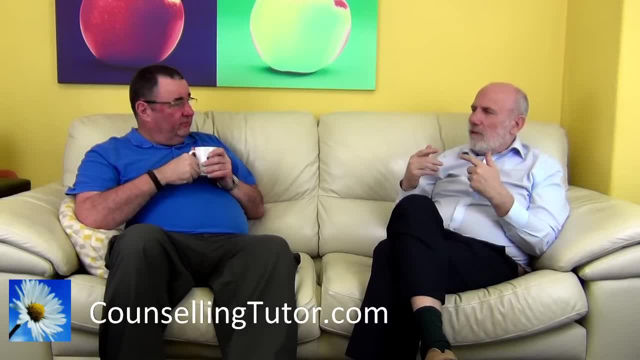 There would certainly be the emphasis on the client understanding those dialogues. the consistent object, Yes, And also the negative, other or the negative objects that they may have internalised at the same time. Okay, Because the problem comes of course not with the internalisation of the good enough object. 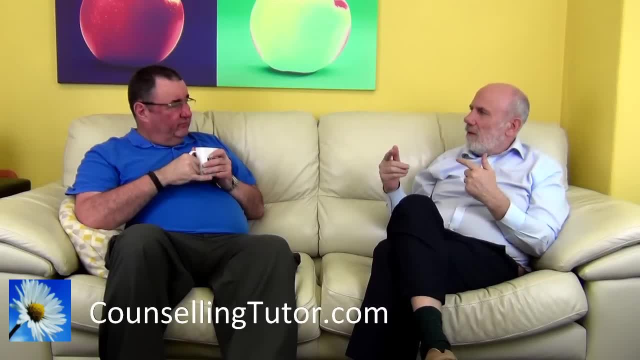 but, of course, if there's a break in the attachment process there, if there's a loss, if the object, if you like, is unhealthy- in terms of if they're an abuser, Yes- Or if they shame the person or if they humiliate the person. 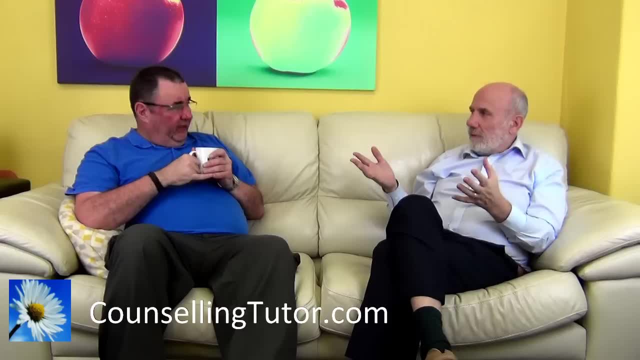 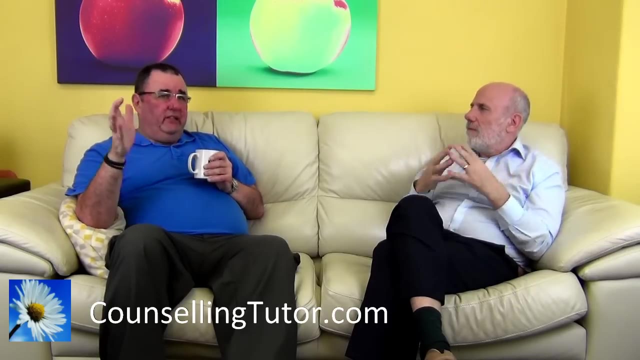 So the object constancy has to happen. Yes, Part of psychological development. However, if the object is, in inverted commas, unhealthy or abusive, then you will internalise that object. Yes, So if you've got a very abusive caregiver. 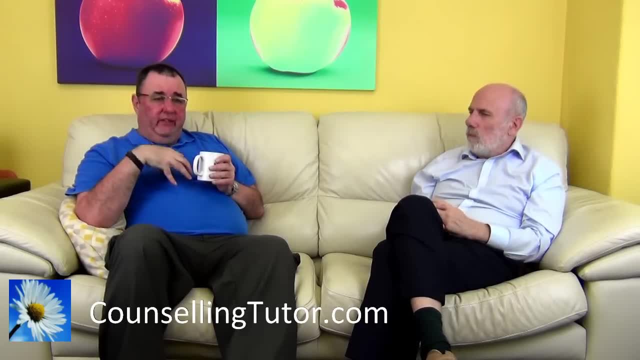 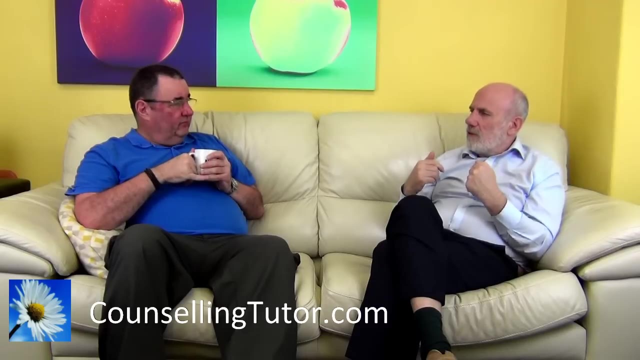 when you're stressed out or you're in a position where you need soothing. instead of the soothing, you will be giving yourself those negative ideas from your past. Correct, And that makes up predictability, consistency, stability in terms of identity forming. 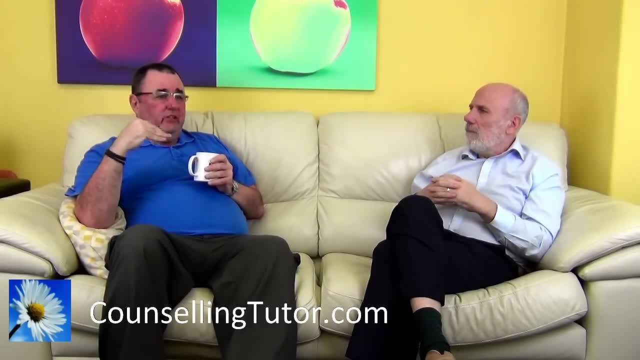 So this is about the formation of personality and how we are in the world. Yes, Yes, And the early objects that make up that personality, Sure. So if you've got a healthy object relation, and it's interesting, isn't it? 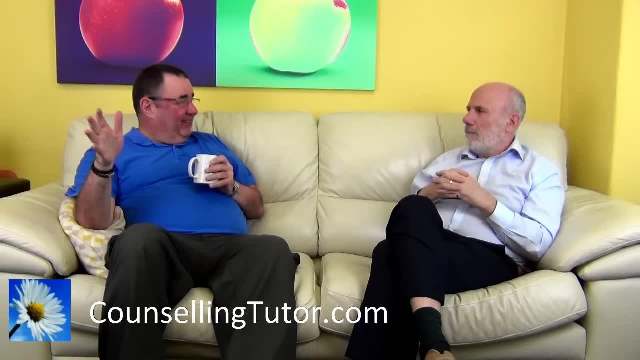 the psychology she talks about talks about mother, But I guess am I right in thinking that that would be any caregiver? Correct, Right, But he was probably a man of his time and chose the mother figure. Correct, But it could be any significant caregiver. 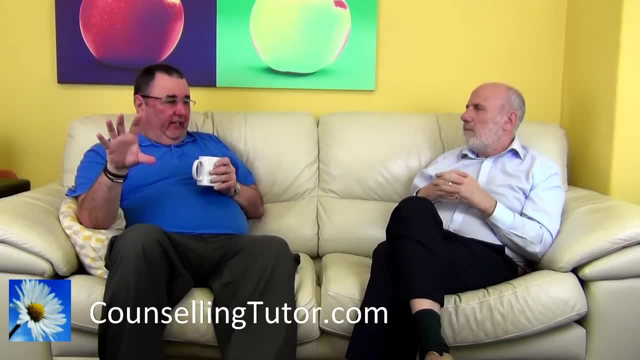 Yes, Cashton talks a lot about that, Right. So if there's a positive caregiver and as someone gets older and they get stressed, they're more likely to be able to self-manage, self-soothe and find a balance in their life. 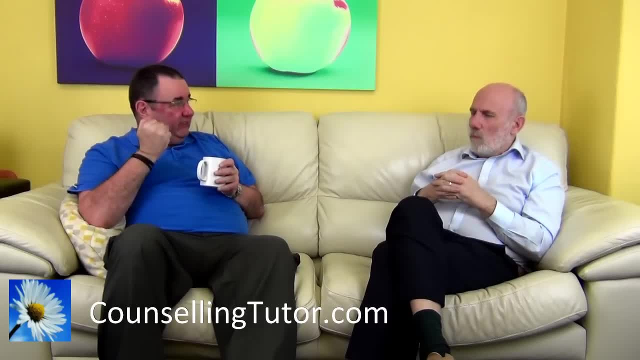 Correct By drawing up this historical object, this historical caregiver. it's like a Jiminy Cricket figure, Correct. What happens when the opposite happens? When the caregiver is a negative force and when the person's stressed, they're pulling this negative force in. 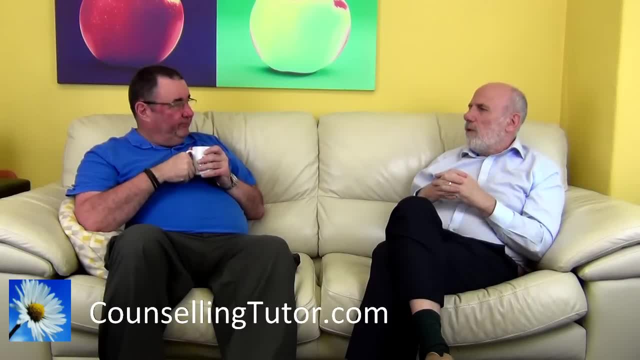 What's liable to happen to an individual? Well, the opposite of the healthy object. Yes, In other words, you will have a negative object, There'll be negative words, There'll be a negative sense of self-image, There'll be a negative sense of self. 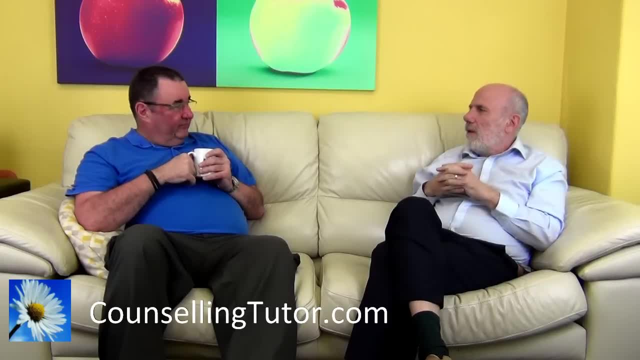 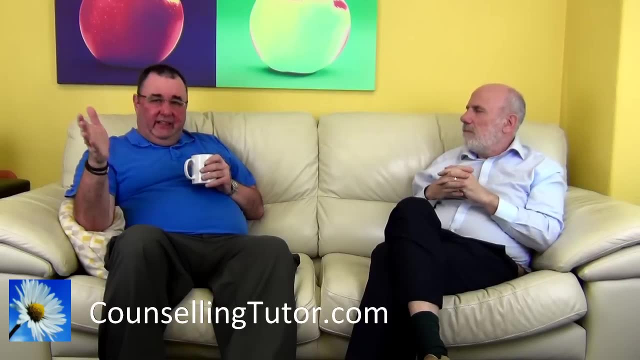 Yes, And your self-esteem will be low And there'll be more what we call unhealth or pathology. Yes, And I think- I don't know if you see this in your practice, but I've had this in my practice where clients have said to me: 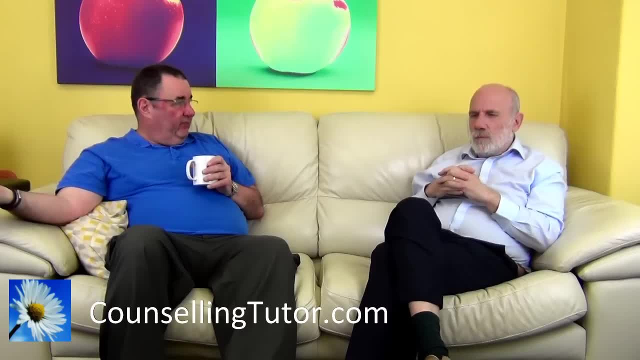 when they've done something wrong, they bring in that significant other from their past, almost like a club wielder to beat them up. a bit more Correct To say: I was told by my father, my mother or my partner, but maybe we're looking at more historical stuff than that. 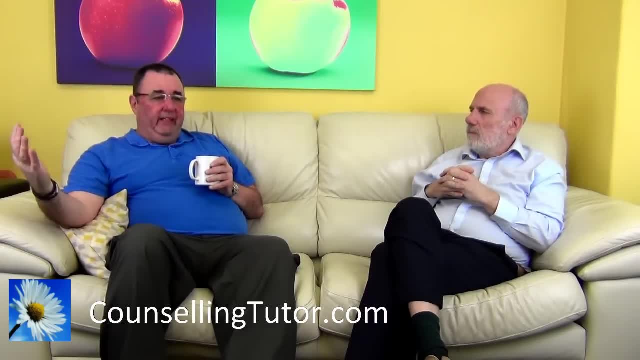 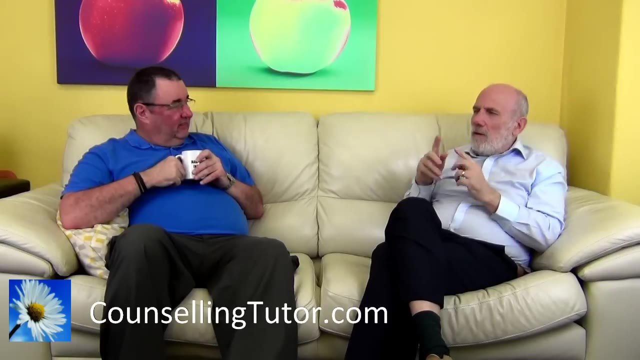 with object relations And they almost seem to make an ally of this person to give themselves a difficult time Correct. So what's the therapist's role in this? Well, now we've come to really the and we can't really talk about object relations. 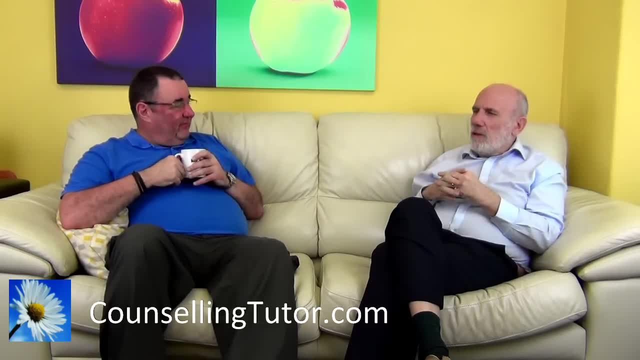 without talking about this phenomena. Right Now, we're really talking about the concept of transference. Yes, Now this becomes very important when we talk about object relations. So, by the mechanism of transference and that is the transferring over the image, feelings, behaviour, 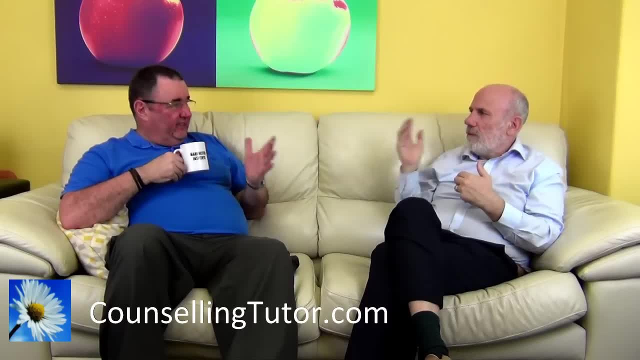 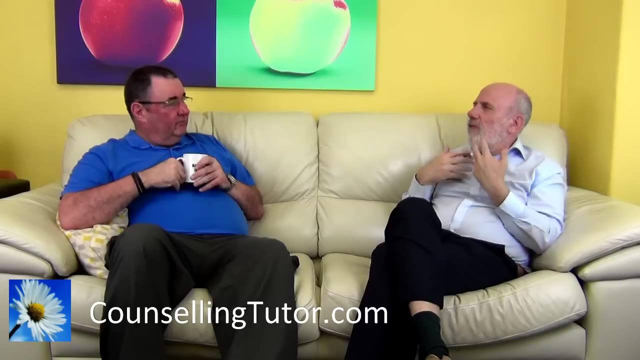 onto the other. that's the therapist's role. Right Presenting past. Presenting past, yes, Yes, That's the phenomena of transference. Through the mechanism of transference, the person can internalise the good object of the therapist. 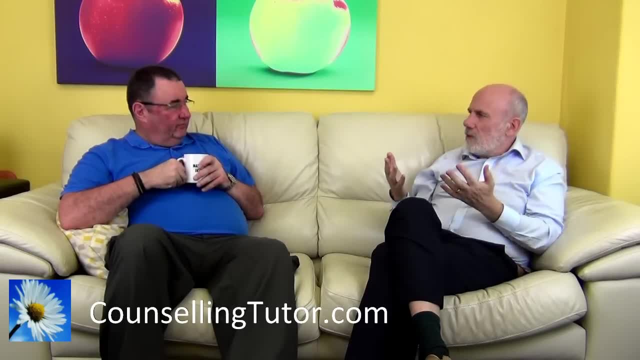 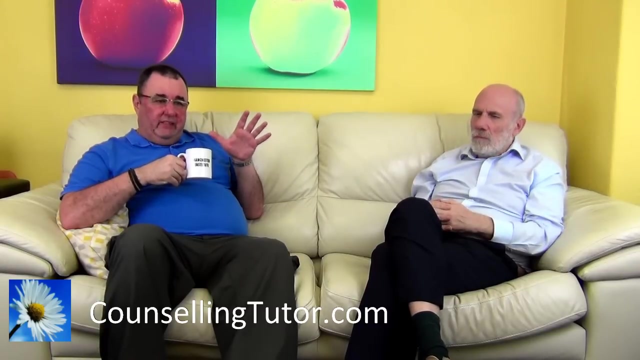 Right Yeah, which will provide protection, idealisation, stability, consistency, close proximity to mediate, if you like, between the good and bad objects. Yes, So that the client can achieve some sense of stability, consistency and empowerment. So it very much sounds like the therapist is another Jiminy Cricket character. 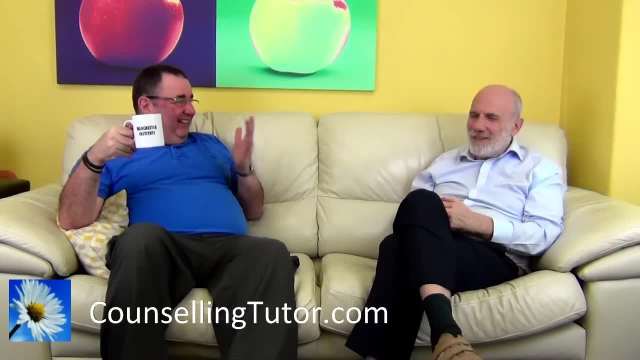 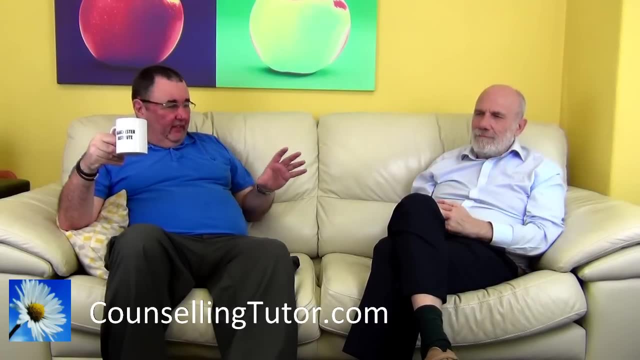 who comes along and, to put it in a better way, Yeah, I quite like that, Yeah. and mediates between this historic object that may be giving the client a bad time and steps in between them almost like a referee, Correct. 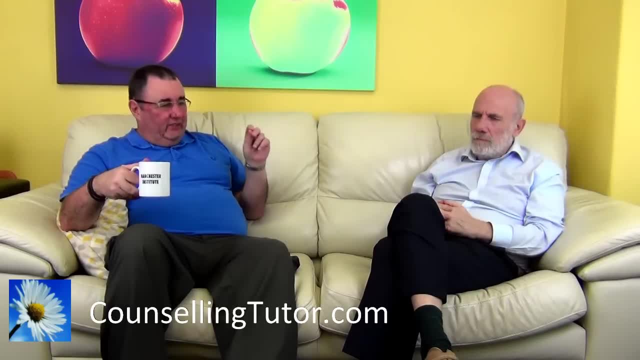 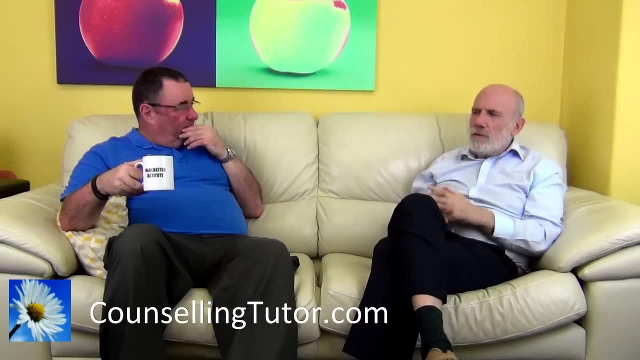 But isn't there something about the fact that this therapist is giving positive attribution to the client? Yeah, there's a couple of things here. Eric Byrne, who was the founder of transaction analysis psychotherapy, coined a term which he called interposition psychotherapy. 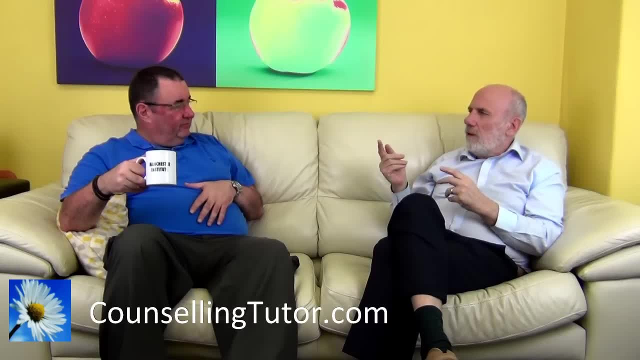 where exactly what you've just talked about occurs: that the client, through the mechanism of transference, internalises the psychotherapist as the good object that will mediate between the internalised healthy and unhealthy objects of the client And in that mediation, 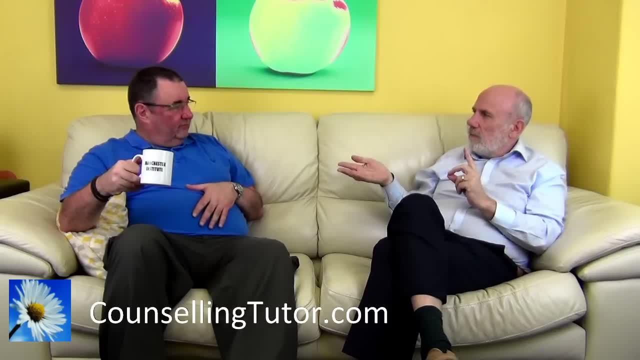 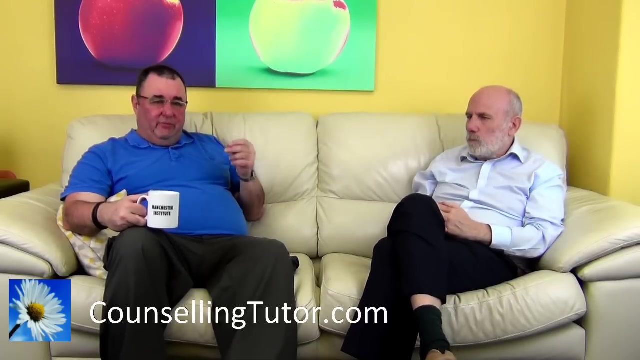 may well give permissions to the client to be able to, if you like, find a voice in the conflict between the negative and healthy objects. Yes, Be able to. you know, there's a wonderful quote by Rogers who talks about the client being trapped in a prison. 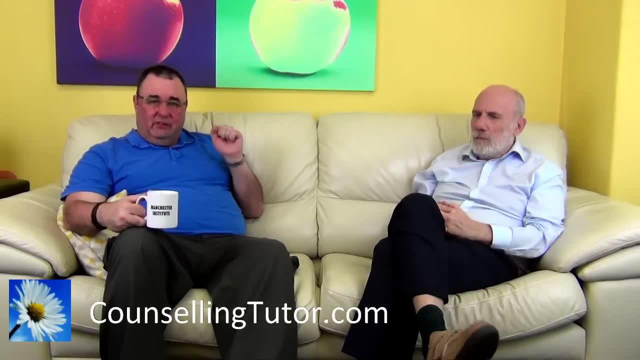 wanting to be heard, knocking on the prison walls, you know, in a metaphorical sense, not literally in prison, And that sounds to me like this. the therapist is helping the client get a voice and be who they want to be, develop themselves. 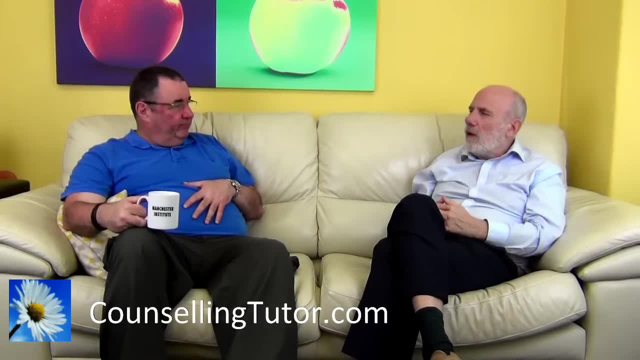 Yeah, Yeah. And Cohert, who is one of the most foremost psychoanalysts, who broke away from Freud in the early 1950s- and it was around the time of Rogers and what was called the self-psychology movement. 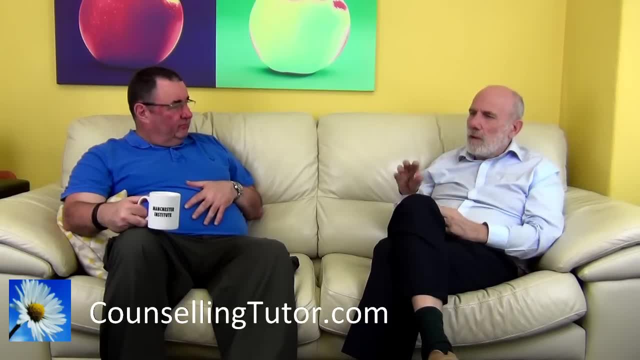 in the United States Coherent three transferences: Idealizing transference, the merging transference and the mirroring transference. And through those particular transferences, then the it's the same again: the client internalizes the therapist. 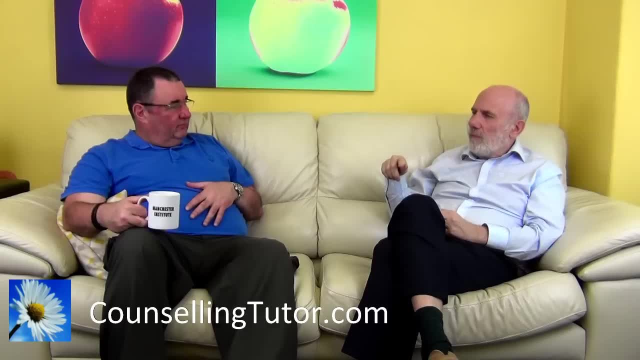 Mm-hmm And the, the protection mechanism through idealization, the mirroring of the good attributes of the therapist, all help the client to develop a more robust sense of self. Mm-hmm Through the mechanism of transference. 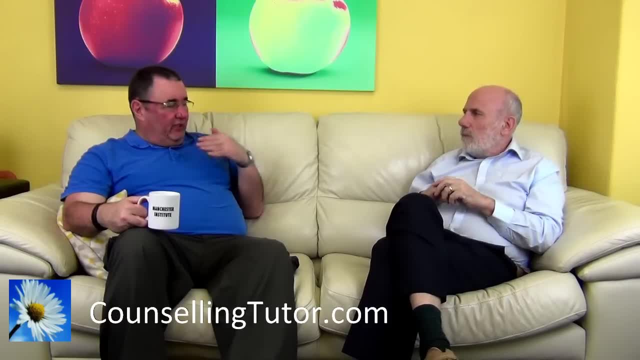 Oh, that's incredible, that isn't it. And a lot of transference is subconscious, isn't it Really? in the realms of unconscious? I mean Freud, way back in his first book on hysteria, when he started to develop the ideas of transference. 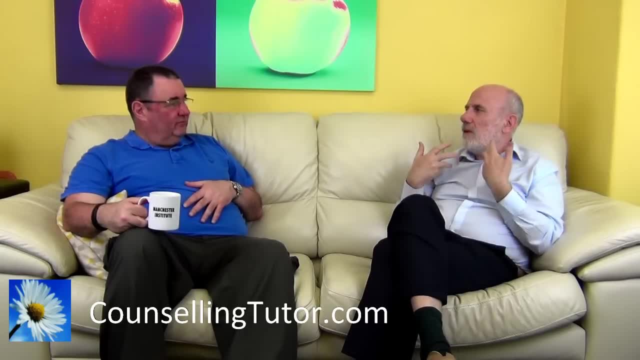 and the use of transference to help this internalized process in terms of object relations that we're talking about, went as far to say, to say a psychoanalysis in terms of a curative effect won't happen without transference. 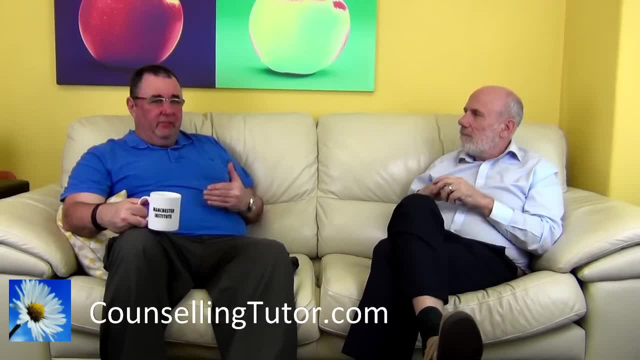 Oh. So there needs to be in this particular moment, in this particular model, the notion that at some level the therapist is internalized to the client. Correct. Otherwise, as Eric Berne said, speaking 60 years later in his model, 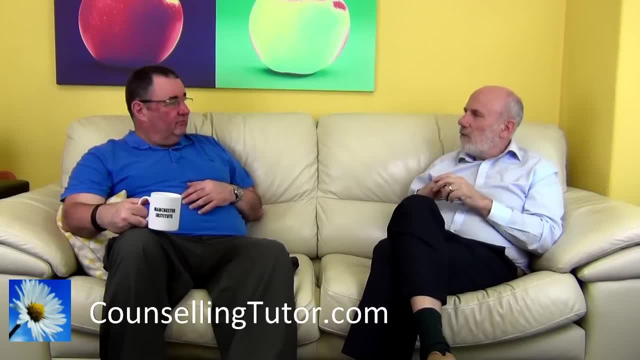 Mm-hmm, you would simply be having an adult-to-adult chat. No cure will happen. Oh, So it has to be more than just a just a chat. It has to be Yeah, So what? what attributes does the therapist need to show? 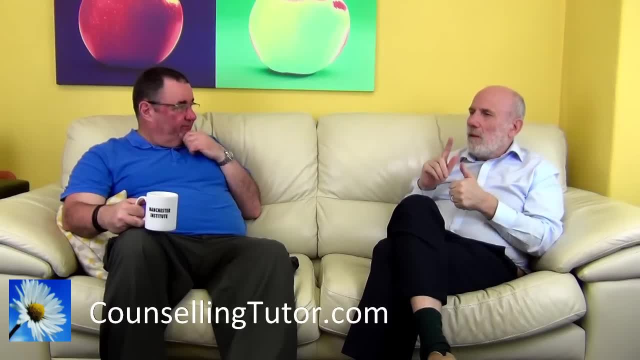 to develop this significant other object: Stability, Mm-hmm, That means always being there for the client. Yes, Consistency, In other words, in terms of mood swings, that they actually are providing a nurturing, a nurturing support, Sure. 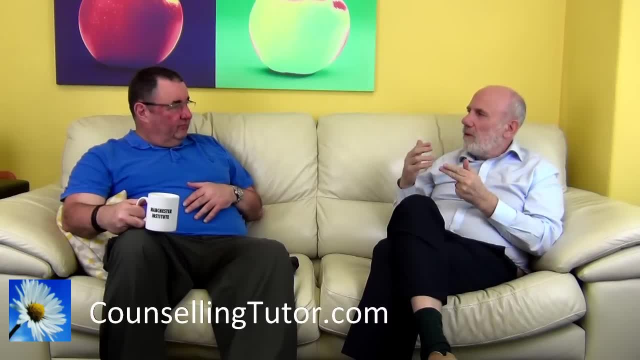 Permissions That they are giving healthy permissions to the client. Mm-hmm. Modeling a healthy enough other, Yes. So all the kind of things that that that therapists should be doing, Should be doing, Should be doing, Yes. 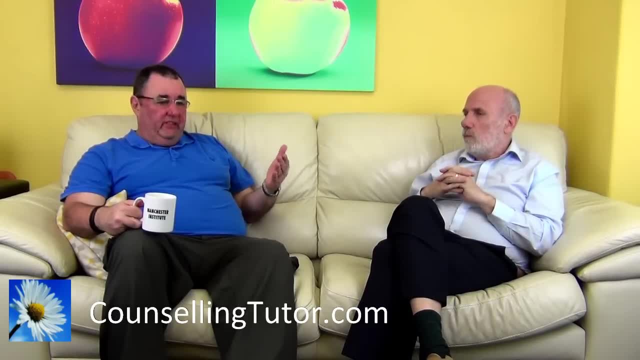 And that's the, that's the key thing here- Should be doing, Should be doing Of of maybe in terms of consistency, turn up on time, turn up prepared for the session. In terms of of giving permission, allowing the client space to explore the material. 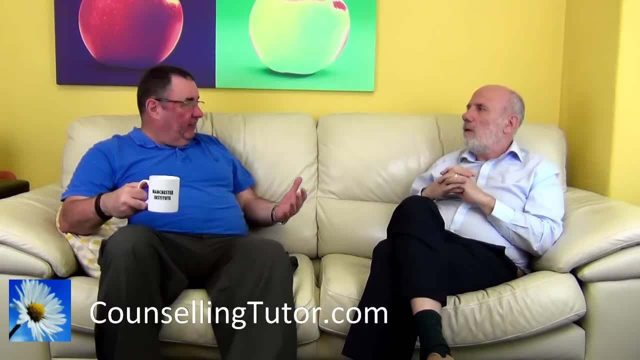 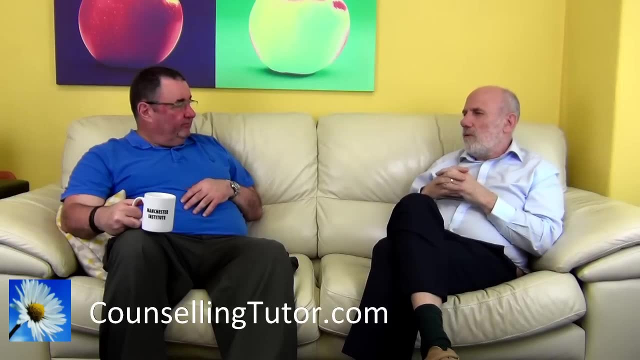 Correct. Yes, And of course it's. it's, and of course again, Cowart came up with the discovery of what he called empathy, A quality which he said that all good in inverted commas. I don't know what he meant by good. 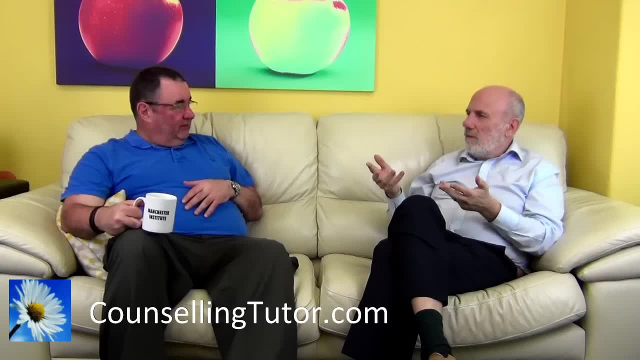 Right. Anyway, psychoanalysts needed to develop Mm-hmm. The ability to get into the skin of the client, Yes. In the service of achievement: Yes, And that will help help develop the mechanism of transference: Yes. 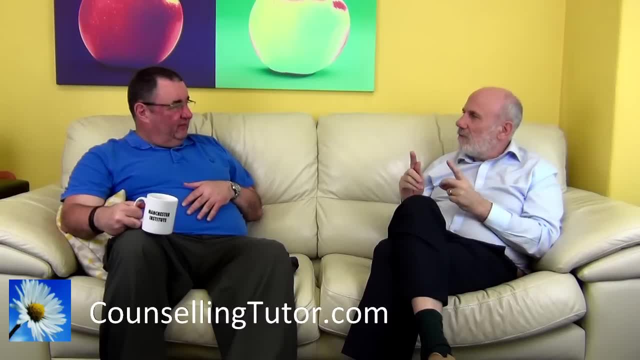 See, it's all going back to this development of transference through basically the unconscious mode really. So it's interesting you talk about en therapeutic, therapeutic in human. Sometimes, when I'm teaching, I talk about internal frames of references. 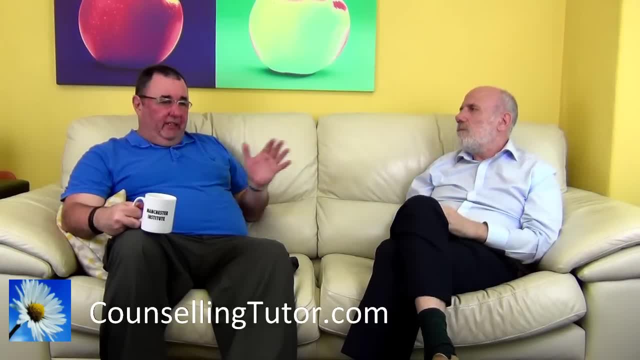 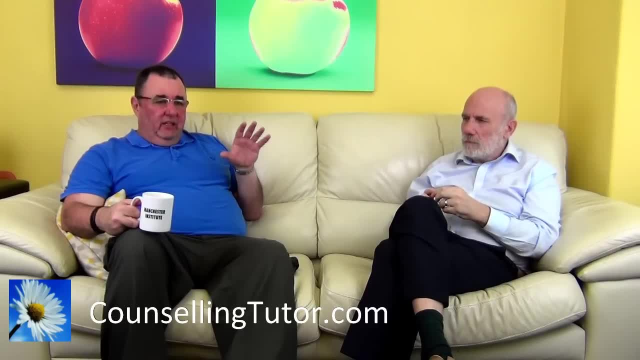 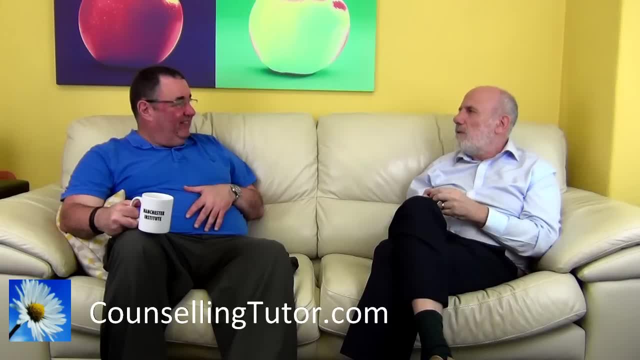 transactional analysis to give some clues into the answer, or at least the response here. Now he would say when the client has developed a robust enough sense of adult over time so that under stress they can organize and regulate their emotions, so they can stay in the here and now. Yes, so they're not catapulted. 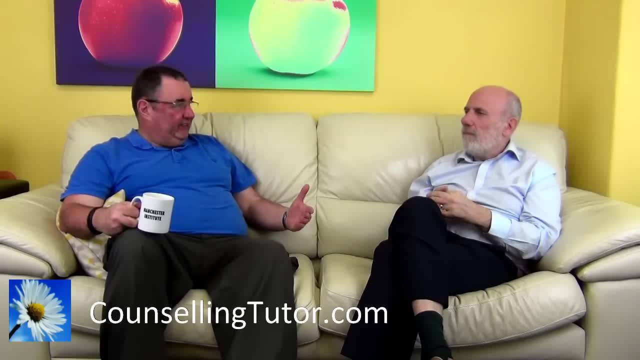 back to the past and that negative object and hearing that negative object speaking to them, as they may be as small children, but they can work with here and now responses and I guess in TA theory, access their adult ego state Yes, and cashed in. speaking about object relations therapy or Kernberg, talk about psychoanalytical 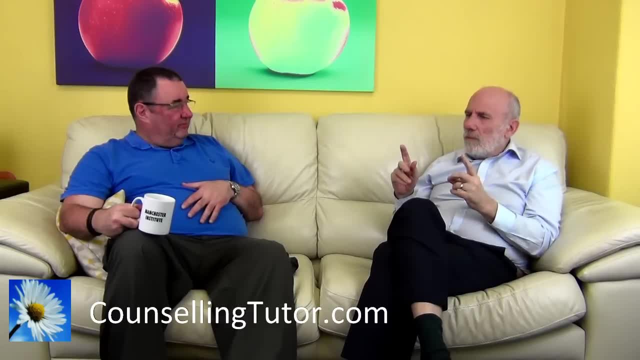 borderline theory would talk about the integration of the negative and positive objects so that the person can mediate between the two and develop their robustness of self. Okay, so know the difference between that negative voice and positive voice and be able to in their own way. 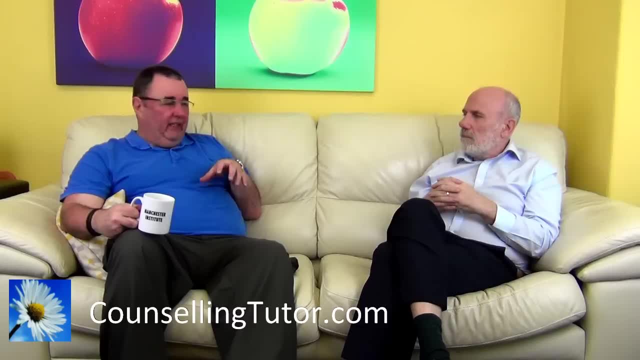 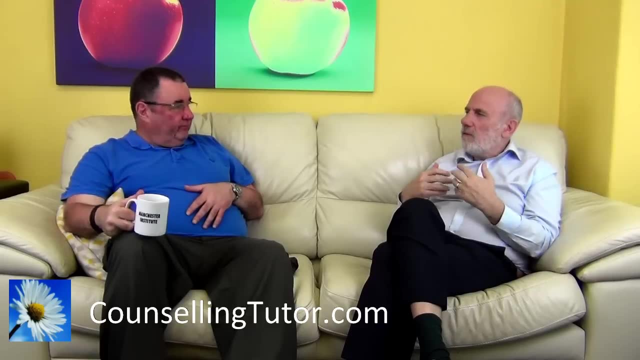 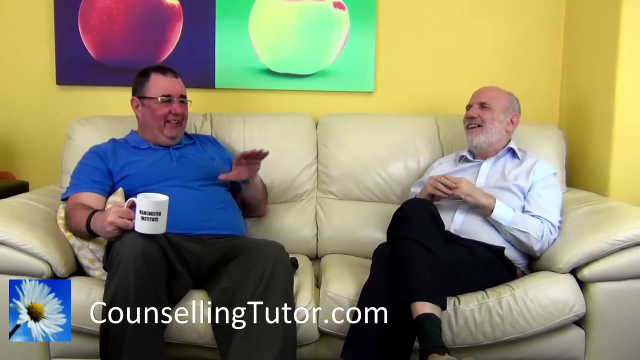 say: actually that is the past, the here and now is completely different, Correct, and I mean that has developed the ability of spontaneity and the freedom of action in the present, instead of being stuck in some archaic child ego state. yes, It's like a bit like the time machine isn't in a way. They're kind of 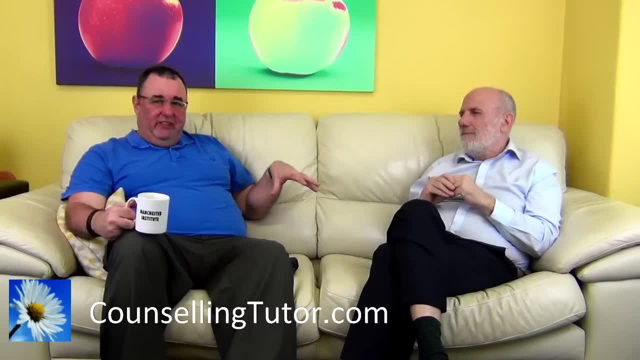 in the time machine, you know, stuck in the past with the feelings, thoughts and behaviours of the past, and then the therapist helps them to come to the here and now, into the present time, and regulate themselves and be able to have that internal dialogue. Yeah, absolutely. 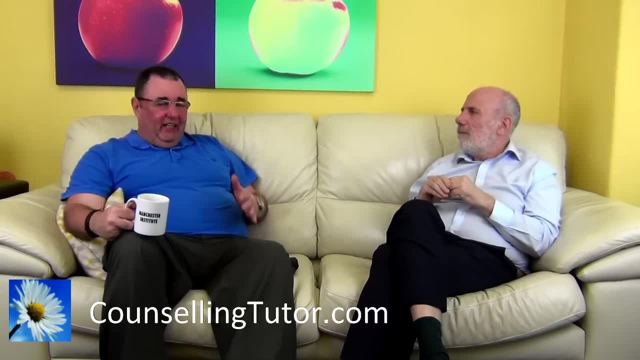 Well, I thought that was really fascinating. I've learnt so much. it's not a subject I have to be honest to say that I know a lot about, and I'm just so grateful for spending this time with you, Bob. I've learnt so much and I'm sure the people who are going to watch are going to learn. 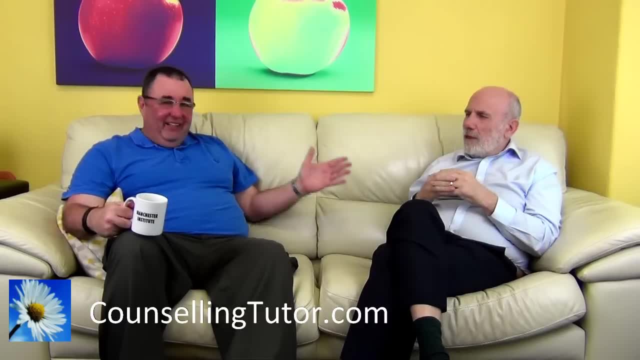 equally as much So Bob Cook. thank you and, as always, to you out there, thank you for watching. Thank you, Thank you, Bye, bye.